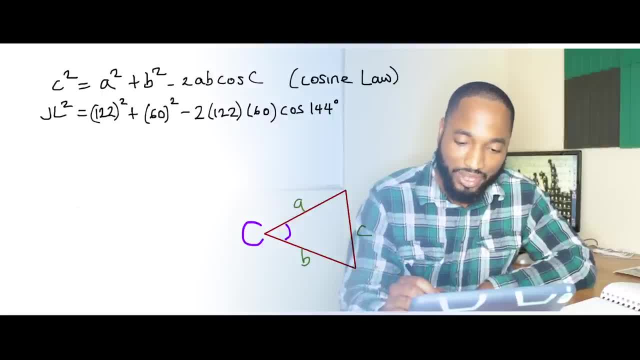 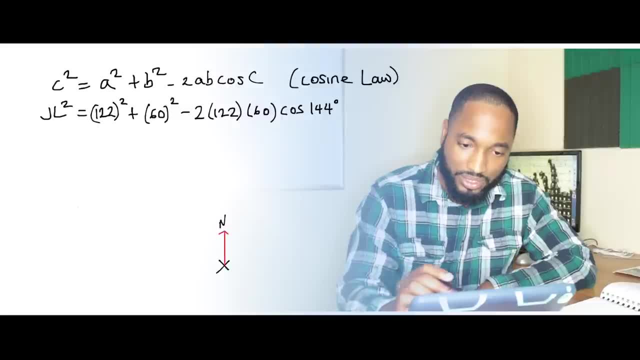 You should already start smelling the cosine. You should already start smelling the cosine rule from a mile away And using that setup, I can find the value of this line here. Now can you see that plane off in our diagram? Let me just skip to where this diagram can be shown. 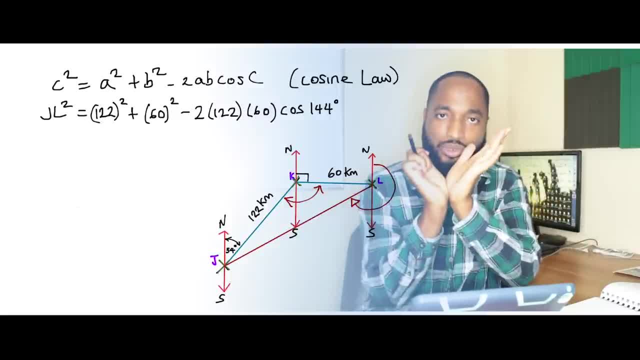 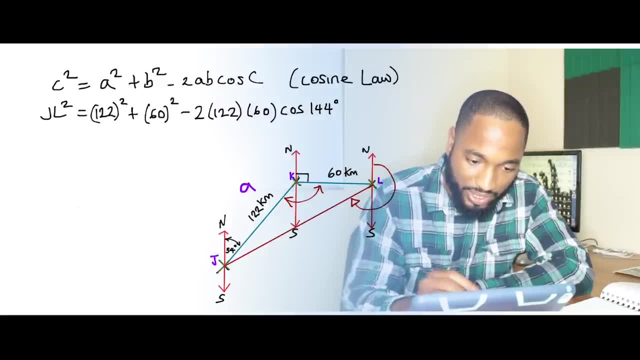 Let's see. Remember what I said: two lines, an angle in between, and we're going to get that line. So we have two lines. I can call this line A, this line B, which is 122 and 60 respectively. 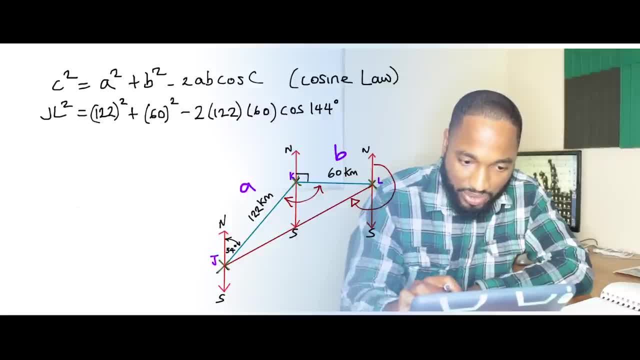 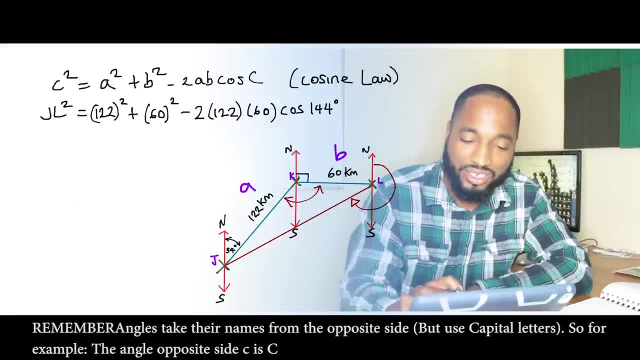 122, 60. 120.. That will allow me to find C, which is JL, And the angle in between is right. here, which I just found, I found that to be 144.. So that's where those substituted terms come from. 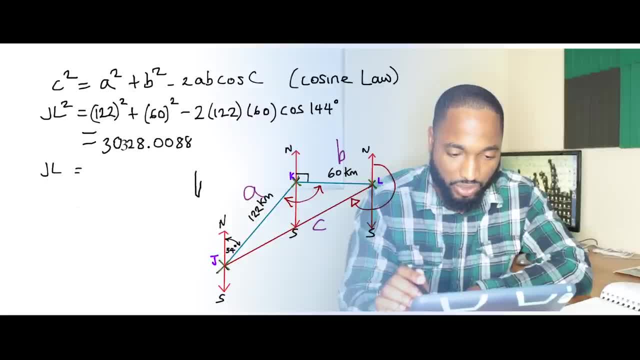 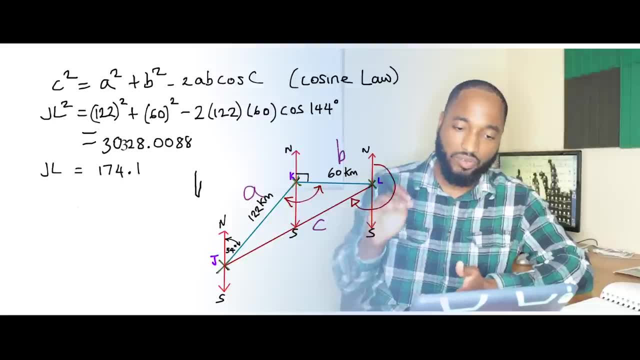 So now I can go on and see, I can go on and record that 122 squared plus 60 squared minus 2 by 122, by 60 by the cos of 144.. Put that in your calculator. Remember the best thing to do, maybe. 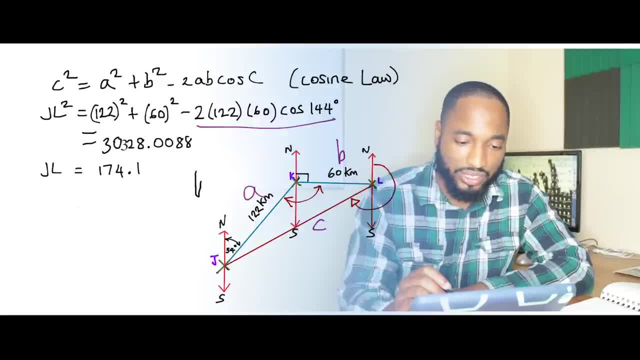 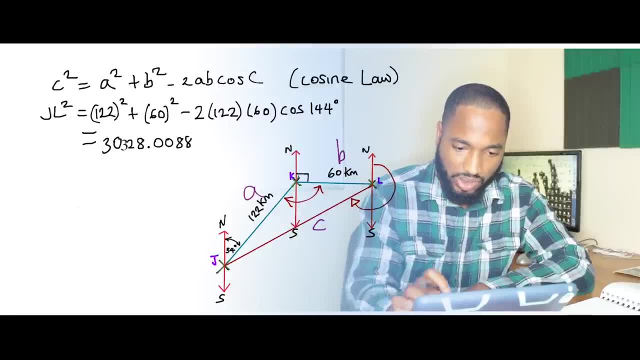 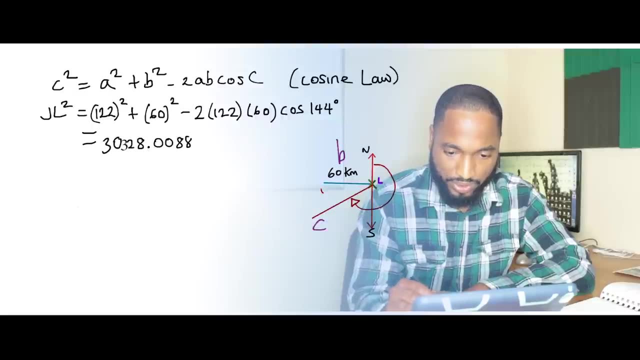 to put this in your calculator: First: record that, Record these two terms and subtract them both. right, All right, All right, So I can just erase this now, Make some room for my working. And erasing, and erasing, and erasing. 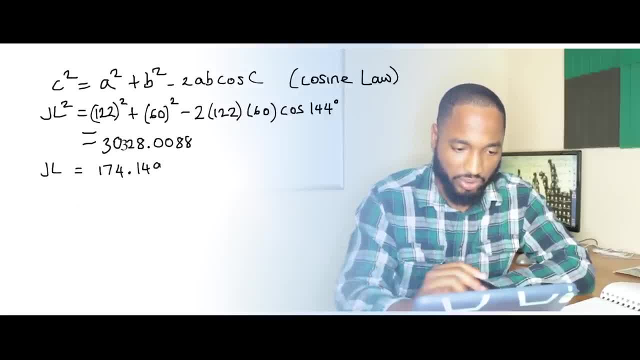 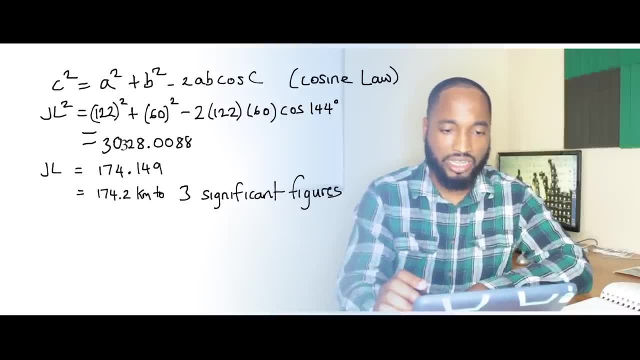 So I can just finish off this question now. JL is equal to the square root of 3028.. You have 174.1449.. Approximately, that's three significant figures. All right, Let's look at the third part before our time is up. 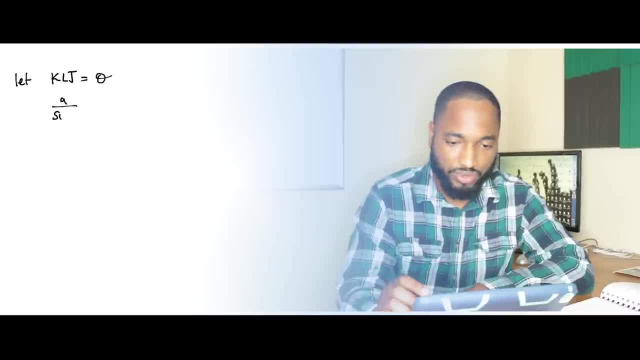 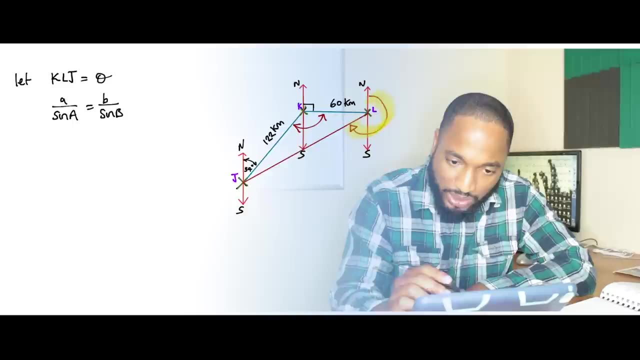 We want to find the bearing now, So I think it would be best for me to just bring back the diagram There. So we want to find this bearing that I'm highlighting in yellow, And the best way to go about finding that bearing is by finding this angle in between. 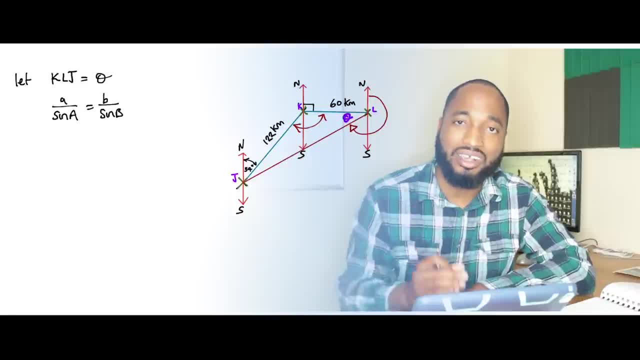 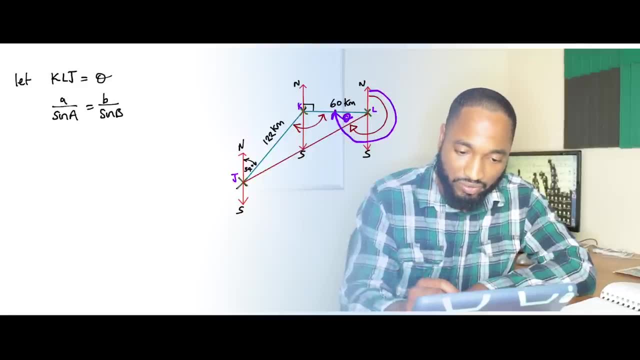 which I'll call theta, And just subtract, Subtracting that angle from 270.. 270 degrees, because this whole thing here is 270 degrees. So if I find theta and subtract it from 270, I'd be able to find the angle. 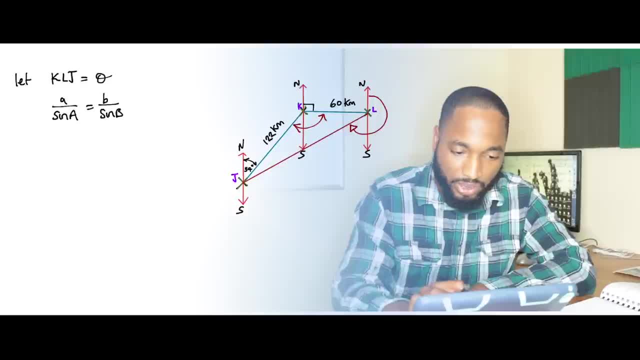 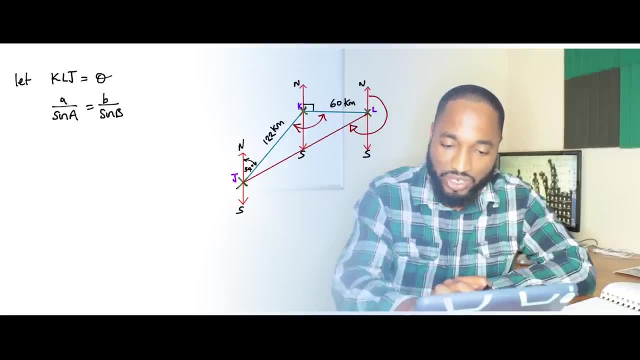 I hope you can understand that there. Take a little look at it. So I'm going to find theta. Theta is really KLG, right? And here's what I have to use. I have to use the sine rule. The sine rule is basically a rule with ratios. 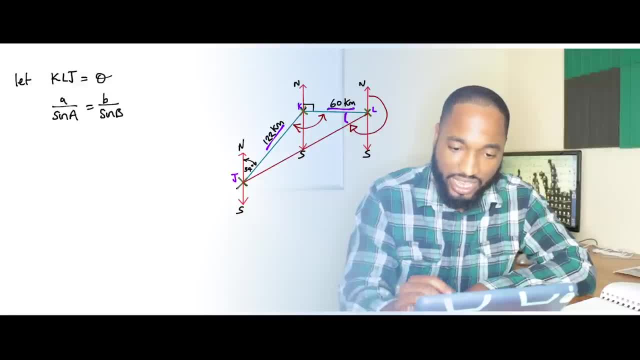 So if I have this side and this angle, this side, and No, not that side, Not that- 60. The side we just found, I forgot what the value was, This side and that angle, here we can therefore use the sine rule. 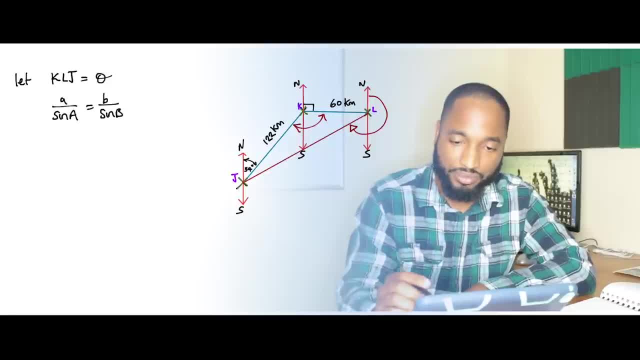 The sine rule is a ratio of the side to the angle opposite. All right, So A to capital A, which is this angle here, And B to capital B. So just substituting those values, 122 over sine of theta is equal to 175.. 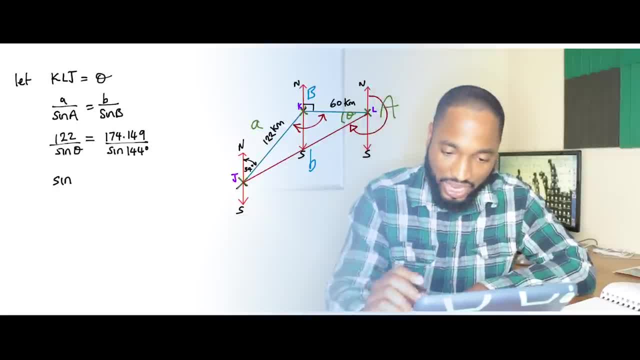 124.149, which is the value we just got for the line over sine of 144.. So I hope you can get that there. I'll just invert the two. I'll invert the two fractions because I want to get theta. 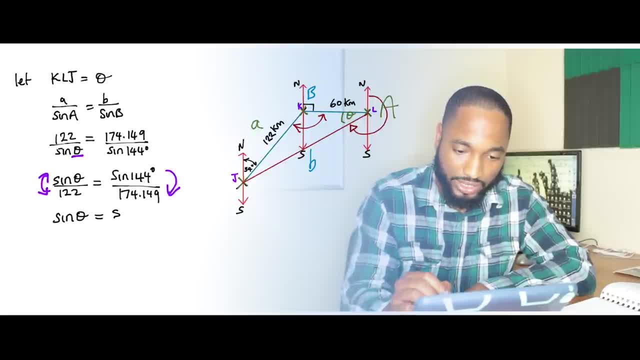 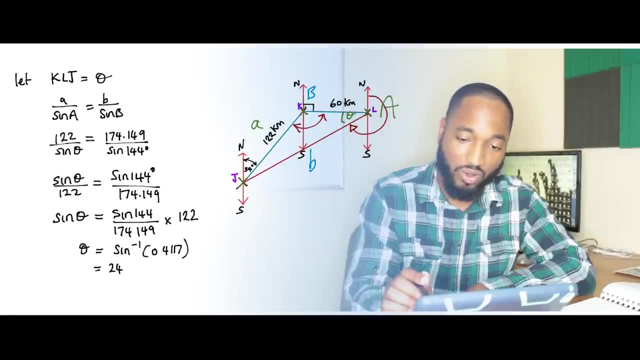 So I'll swap them on both sides there So I can get theta on top. Then it's just a matter of algebra and arithmetic bringing across the 122.. So it'll turn to multiple And therefore theta is equal to the sine in place of all that stuff, which is 24.31.. 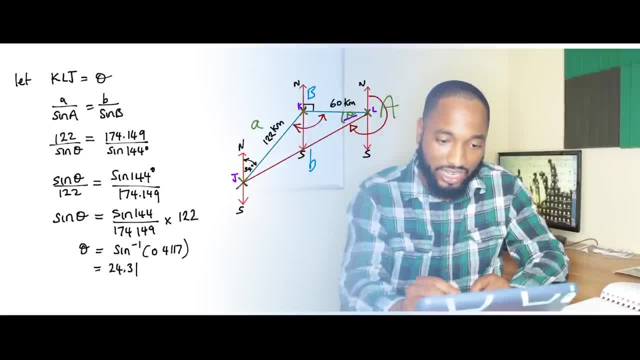 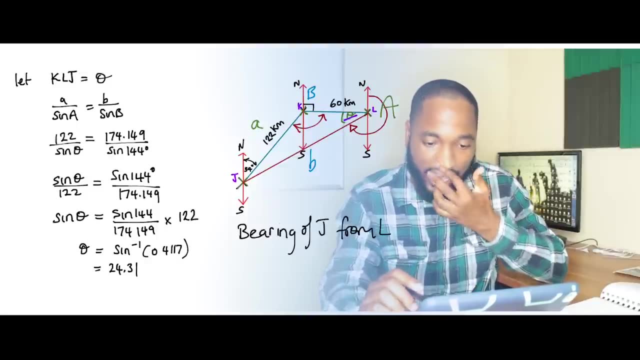 Don't stop there. That just means we found theta. We just found this angle here, 24.31.. To find the actual bearing, we would need to. Where are all these lines coming out from? To find the actual bearing, we'll need to subtract that from 270 degrees. 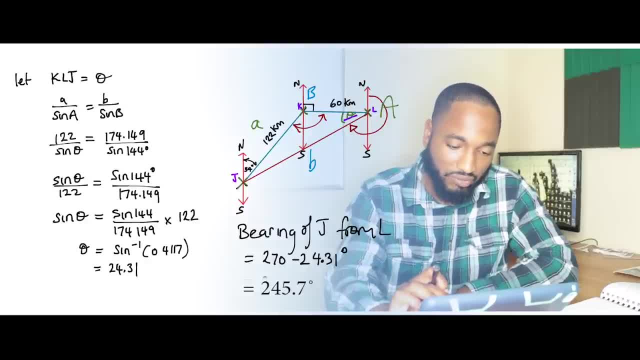 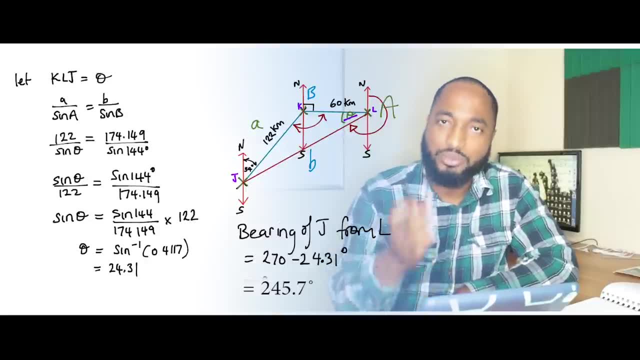 So 270, take away 24.31. And we get 245.7 degrees. All right, I feel like I was a little all over the place in this, But I hope you can just pull back the video and just take it in a little more if you're having problems with this type of question. 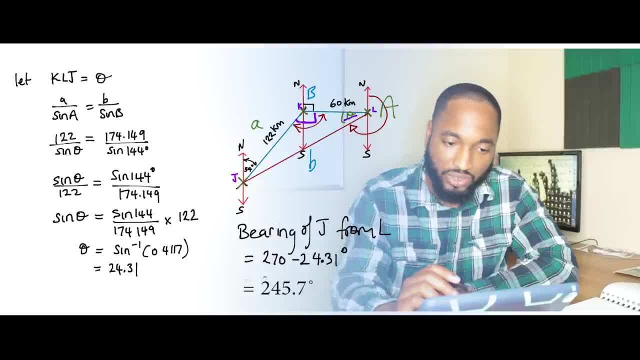 Remember, the first one was easy to find: 90 degrees plus this angle which is alternate to the angle given, 54. And we found JL by using the cosine rule. And finally we found this angle here, theta, by using 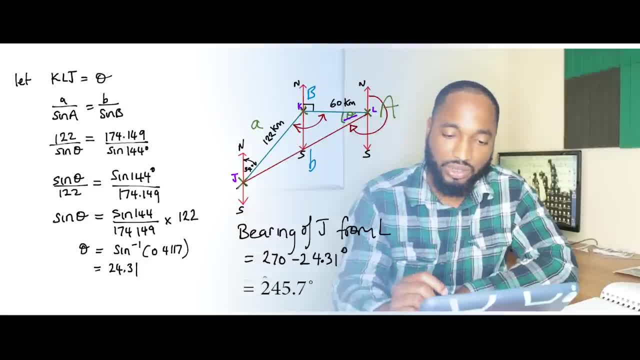 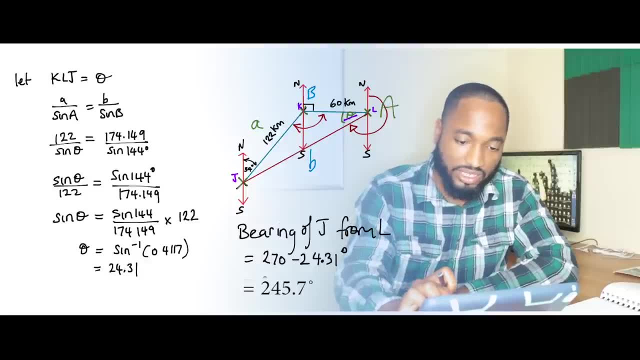 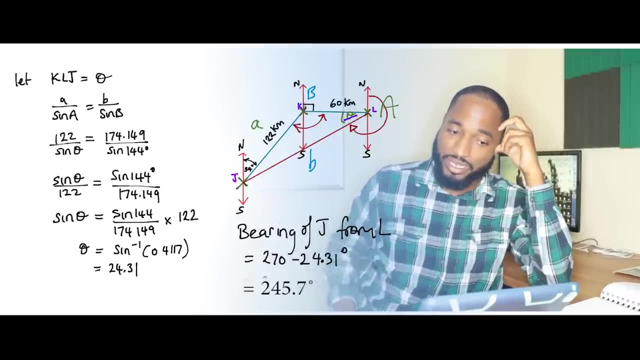 the sine rule And we took it away from 270 to find this bearing here. All right, And that's the last three parts of the question. It goes for seven marks. That's like the toughest part and tricks for you there for maths. 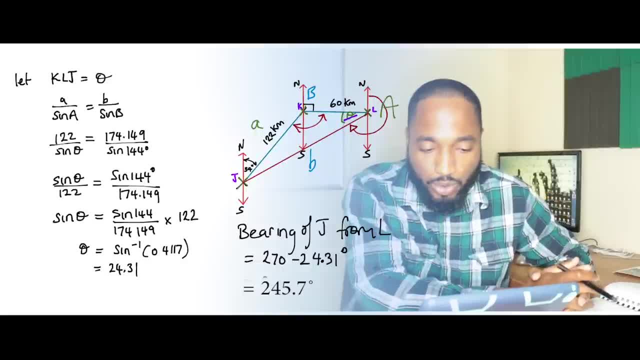 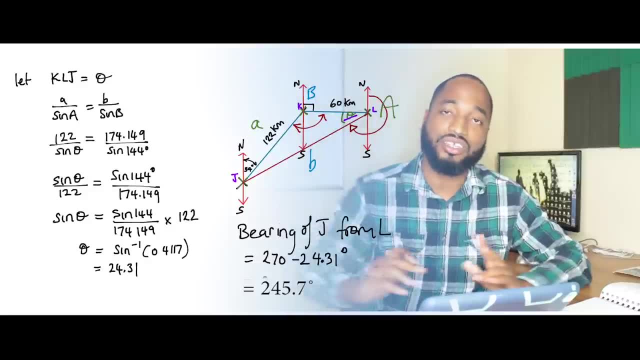 So I hope that kind of shed some light on that for those who asked about this question- this exact same question, And you're able to walk through it by yourself. So go back and check another bearings question And see if you can do it. 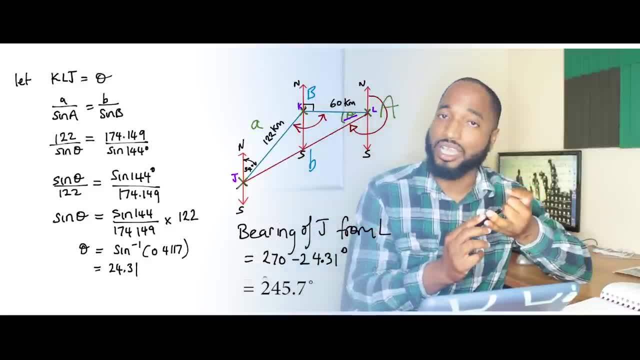 Remember cosine rule sine rule going to play a key factor most of the times in bearings questions. All right, Till next time, Pew. 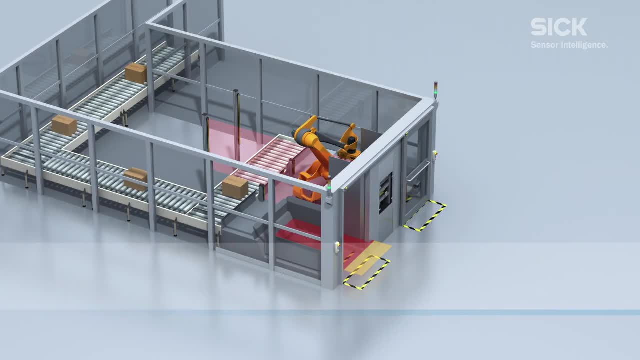 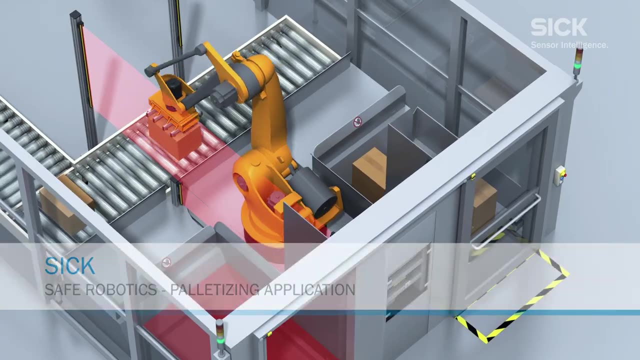 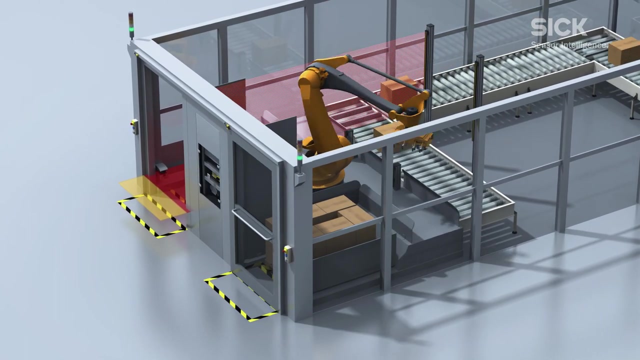 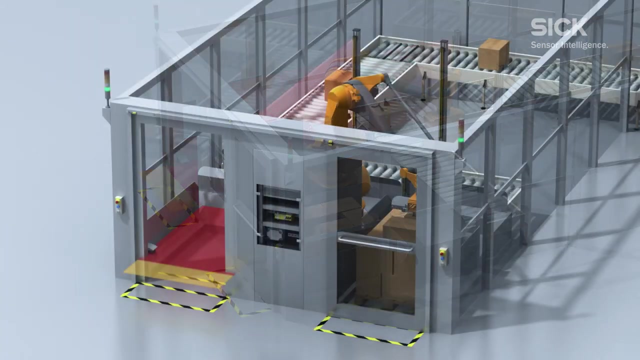 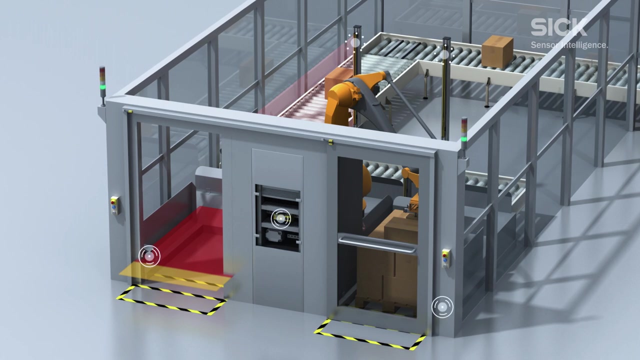 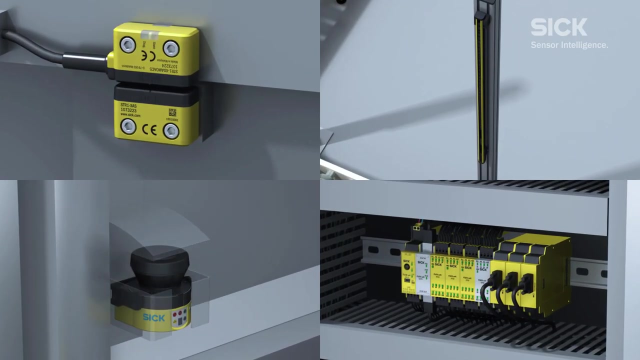 Thanks to SICK Technologies and safety expertise, humans and robots can work together safely, effectively and efficiently In palletizing applications, for example. combining the right safety technologies makes human-robot interaction possible. An S300 mini laser scanner combined with the FlexiSoft safety controller, the DTEK4 core light curtain and the STR1 non-contact safety switch monitors the open access to the machine. 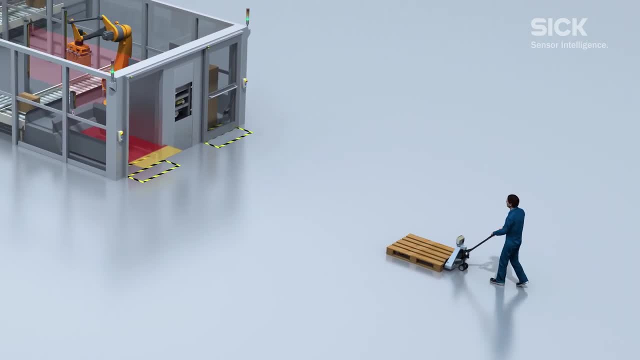 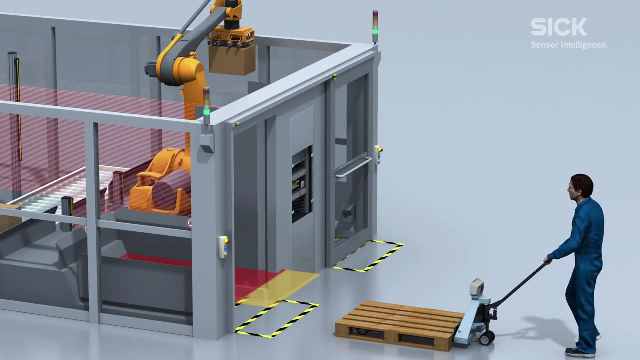 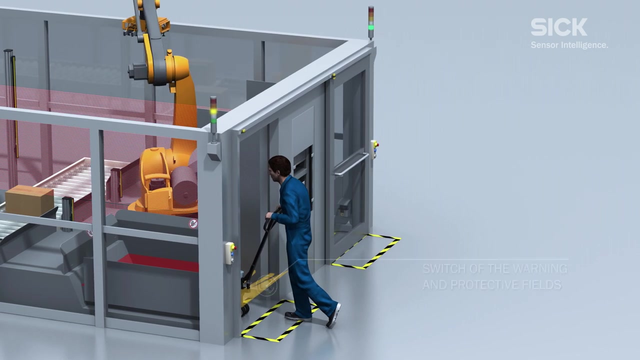 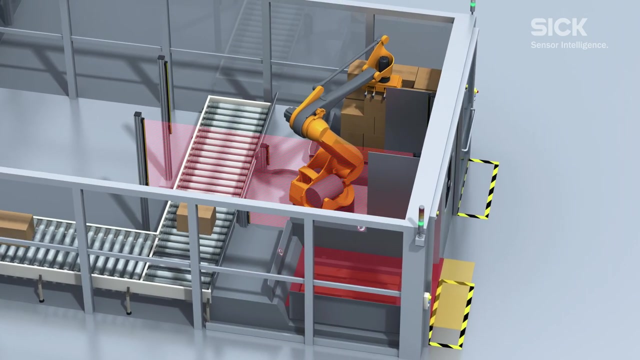 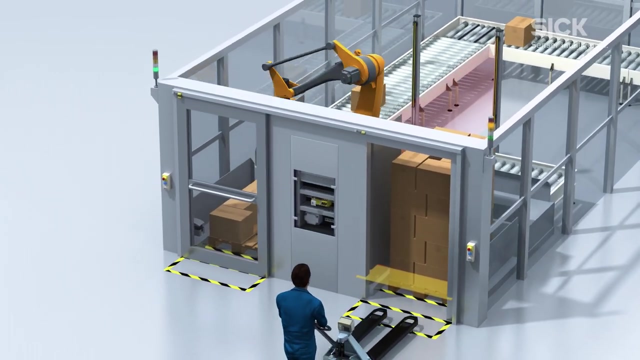 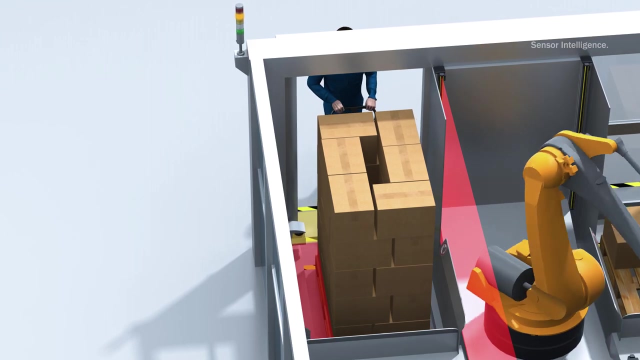 This facilitates permanent interactive production, protecting the operator from the dangerous fast movements of the robot Without using any physical guards. a pallet can be positioned safely in the machine While the robot carries on working, ensuring maximum plant productivity even in compact areas. Additionally, it provides the operator with the ability to monitor the environment. 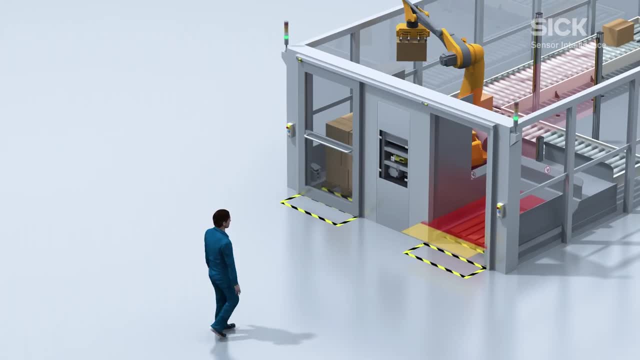 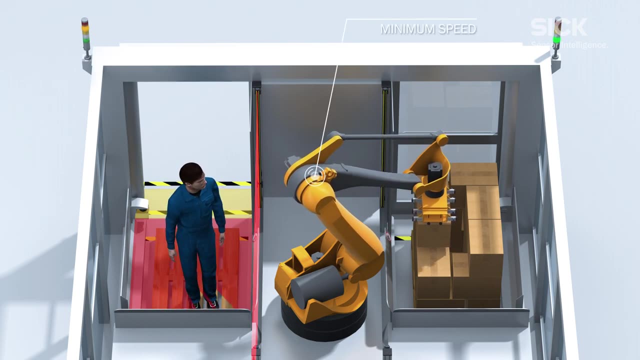 Additionally, it provides the operator with the ability to monitor the environment. This prevents risks for the operator of getting injured by accidentally accessing dangerous areas. If a person unexpectedly enters the machine, the SICK solution enables gradual reduction of the robot speed and a speed increase again when the operator leaves the dangerous zone. 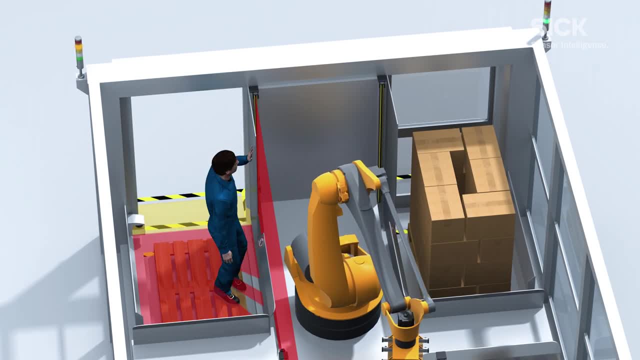 And if someone gets inside the machine, the DTEK4 core light curtain prevents any contact with the moving robot, which is stopped immediately. And if someone gets inside the machine, the DTEK4 core light curtain prevents any contact with the moving robot, which is stopped immediately. In addition to safety and production processes, the combination of the compact safety components from SICK allows you to make the most of the space in your manufacturing area. In addition to safety and production processes, the combination of the compact safety components from SICK allows you to make the most of the space in your manufacturing area.